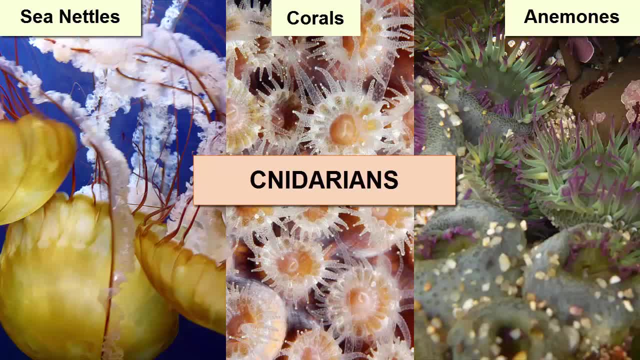 Now let's look back at those eggs. Let's look at those cnidarians and their stinging cells. How do they work? Do all cnidarians really have a sting? Anemones as well? Yes, they do, and here's how it all works. 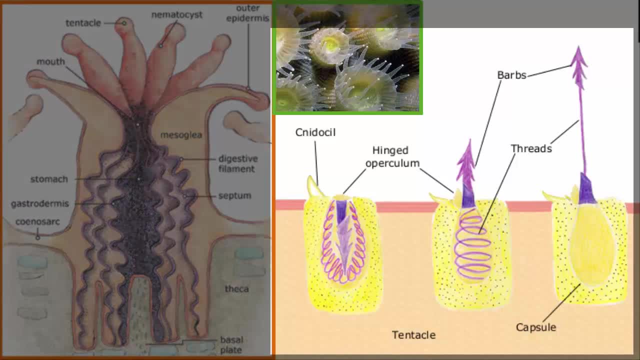 Cnidoblasts are cells with a hair trigger and a capsule containing an inverted coiled hollow thread. Some threads have tiny barbed blades and sharp tips with toxin. Once used, these barbs are discarded and replenished with a new one. 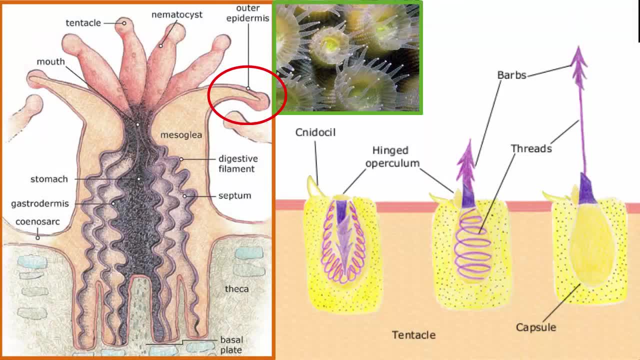 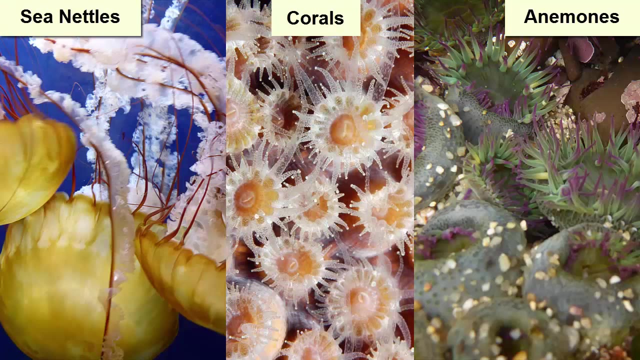 Stinging cells are deployed on tentacles that bend or retract to the mouth. When the tentacles and barbs entangle prey, the cnidarian draws the tentacles back to its mouth and deposits them into a sac-like digestive cavity. These stinging cells are a part of all cnidarians, be they anemones, corals or jellyfish. 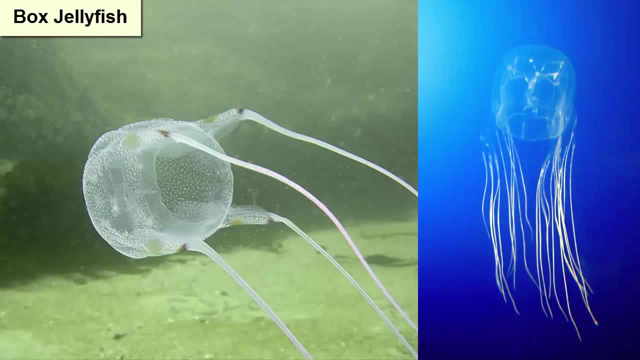 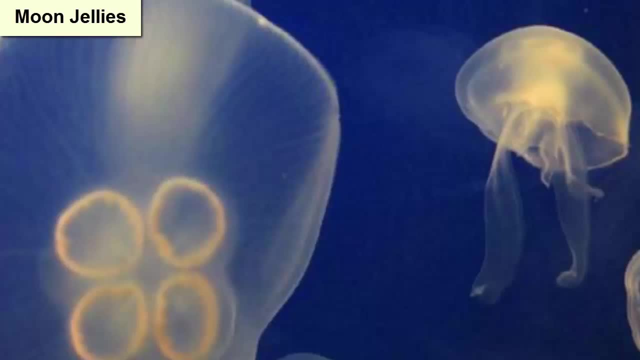 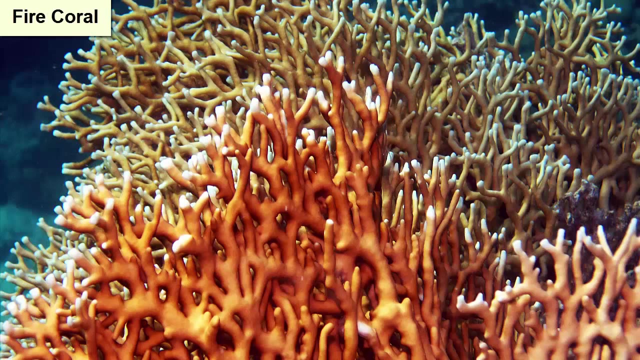 Some toxins are so potent they can kill a human, such as the toxins of the box jellyfish. These are too weak to penetrate human skin or have weak toxins that we can barely feel, such as those of the moon jelly. Fire coral is a species of coral that has a particularly painful sting. 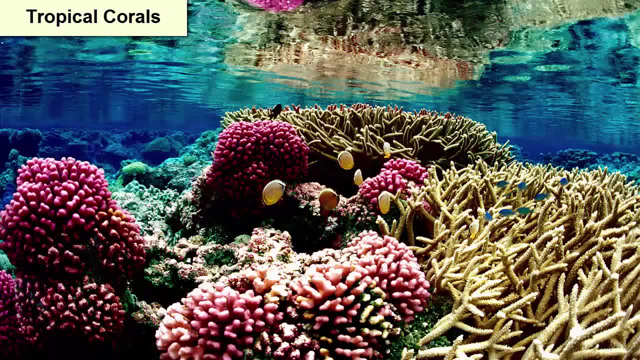 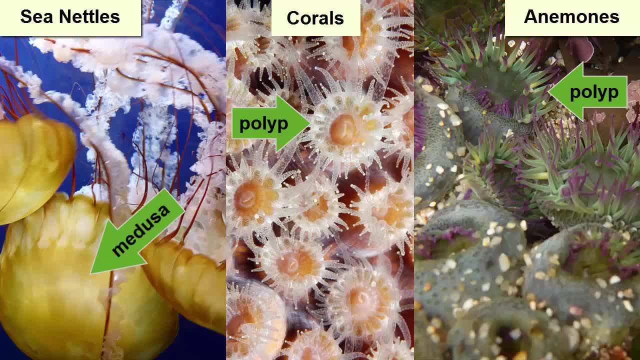 However, most tropical corals are not toxic to humans. Corals and anemones are both considered the polyp form. Jellyfish are medusa forms. What that means is that corals and anemones are similar to jellyfish, but stuck upside down on a rock. 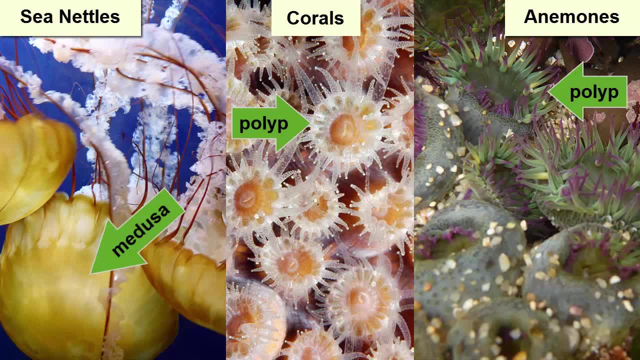 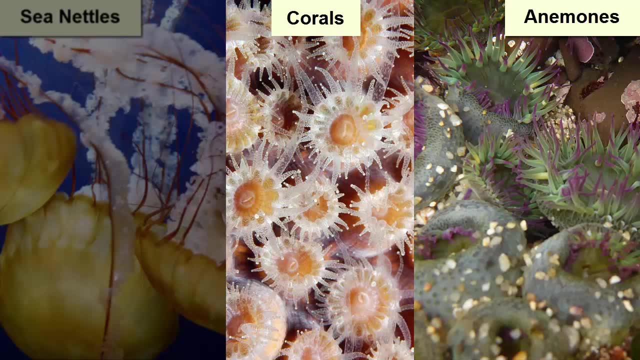 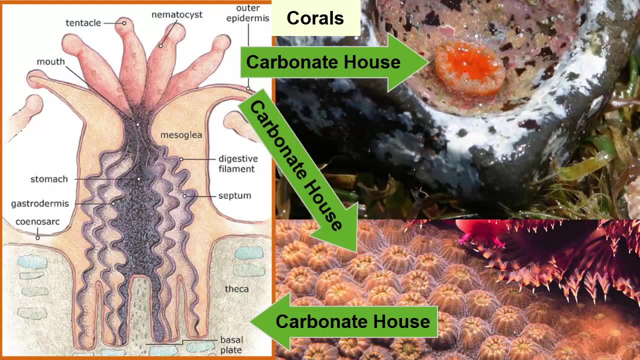 and jellyfish are like anemones that have been freed from the rock and allowed to swim. How can you tell the difference between anemones and corals? They're both polyps and they both form clone colonies. However, almost every species of coral lives in a calcium carbonate housing. 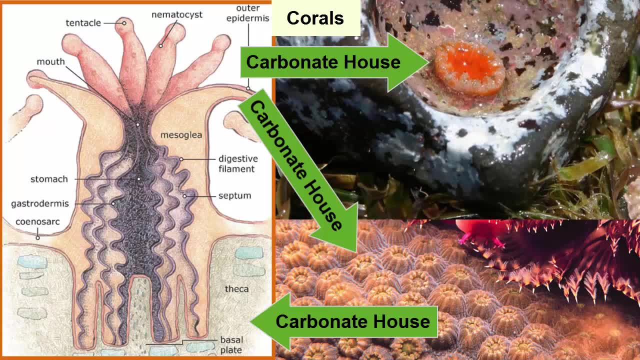 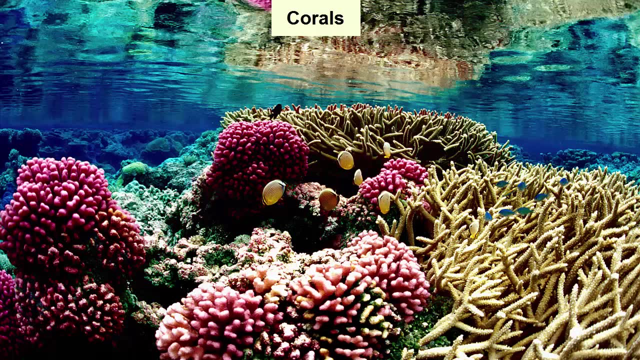 Anemones do not. These houses build up large structures in a variety of shapes, each filled with a clone that has budded off the original. All these different coral clones are connected to each other, not only by their houses, but also by their tissue. 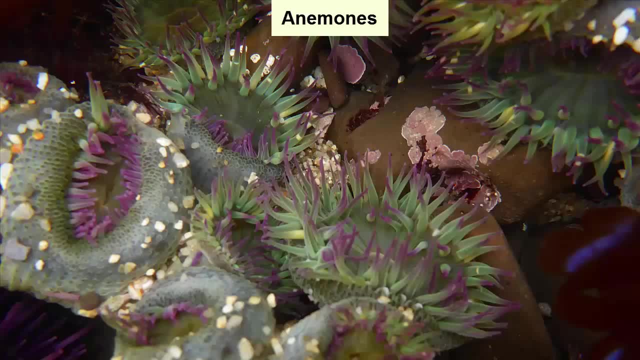 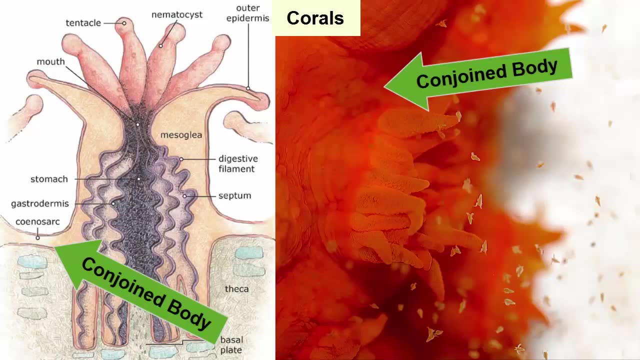 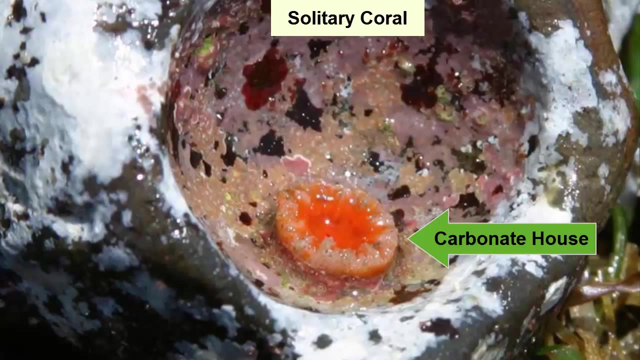 Cloned anemones do not have houses nor shared tissue. This picture shows one of the rare corals that, while sharing tissue, does not build itself a calcium carbonate housing. This image shows a solitary coral common along the Pacific coastline. It has a calcium carbonate house but is solitary and has no cloned neighbors. 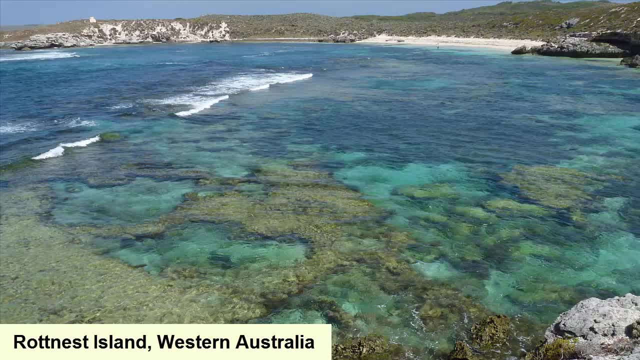 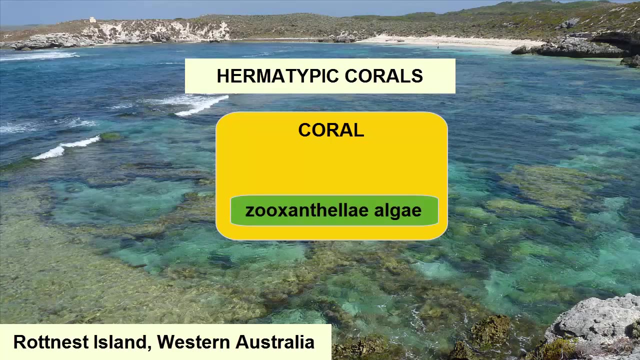 Tropical corals, like those found in this reef off of Western Australia in the Indian Ocean, are hermitipic corals, which means, as discussed in the Living Ocean lecture, they are mixotrophs. They participate in a mutualistic relationship with small dinoflagellate algae known as zooxanthellae. 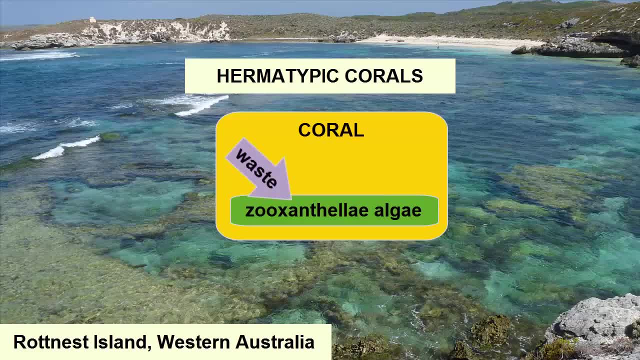 The waste of the coral fertilizes its garden of zooxanthellae and the garden feeds the coral. These types of corals require clear, warm, salty water. Sunlight must penetrate deep enough to reach the reef so the algal gardens can photosynthesize. 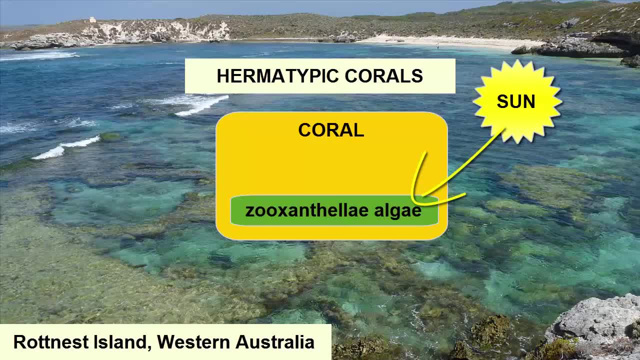 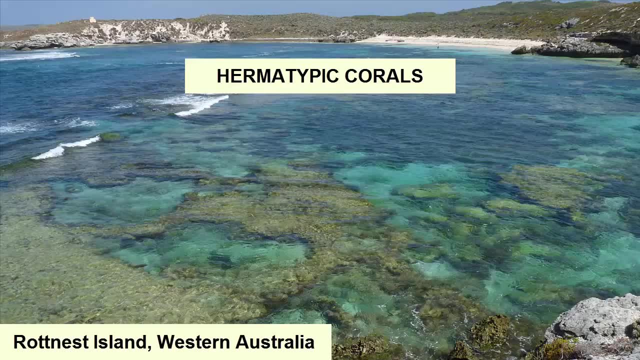 That means the water must be clear of suspended particulates and plankton, So these reefs form where there is no nearby river and the waters can contain a constant warm temperature. In addition, since corals are sessile, they need a solid surface on which to attach. 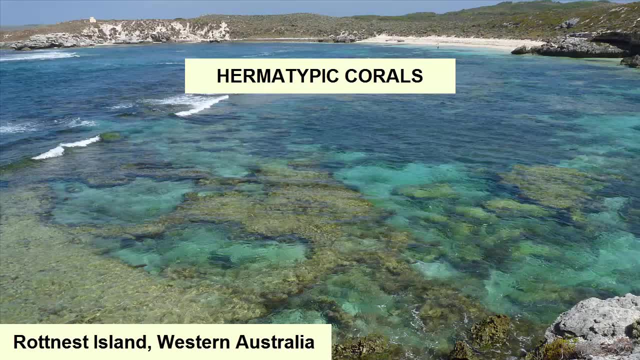 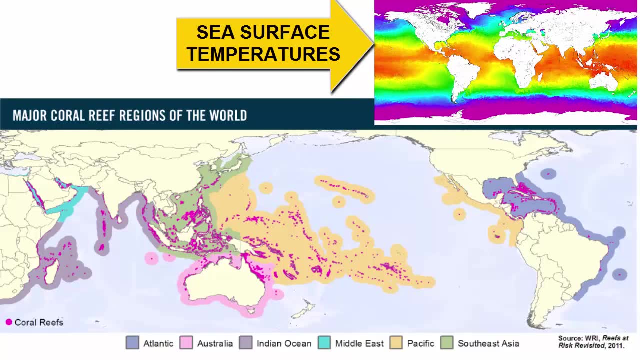 so they need hard rock or other material. They cannot attach to mud or sand. As a result, we find these coral reefs only in tropical climate zones, generally on the western edges of the equatorial sea. Why What happens in the eastern equatorial oceans? 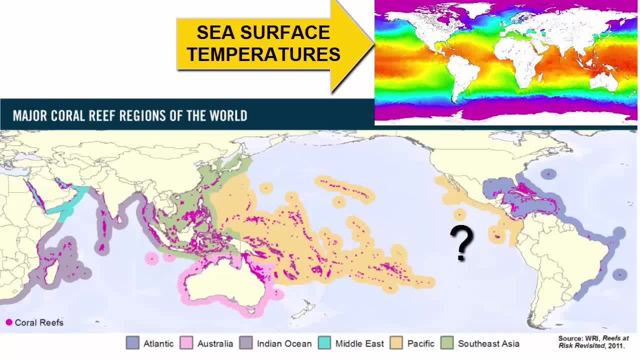 As you recall from our previous lectures, the eastern equatorial oceans alternate between upwelling and downwelling based on the strength of the trade winds. That type of fluctuation would kill a coral reef And nutrients bring plankton, which means a reduction in the photic zone. 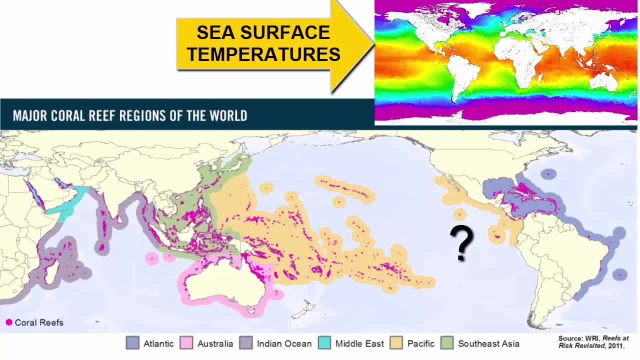 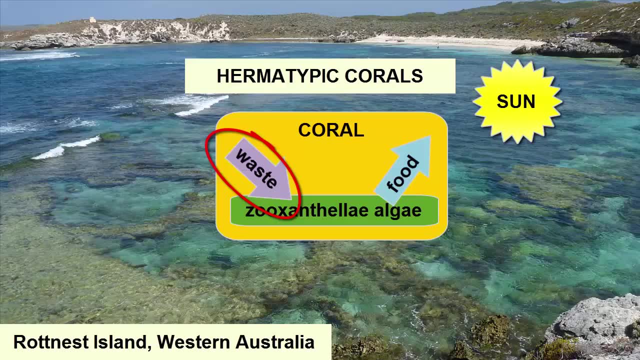 Ironically, coral reefs can survive only where there are no nutrients in the water. So where do the autotrophs get their nutrients then? The waste of the coral? Coral reefs are truly oases in marine deserts, self-contained and sustaining ecosystems.